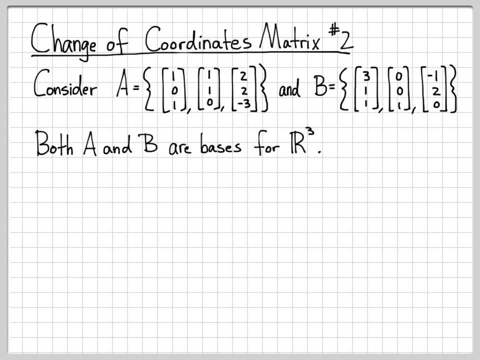 of these are bases for R3.. You could check that there are indeed three vectors in each of these sets. That's pretty obvious. And these vectors are linearly independent, So dependent, so they span R3.. So these are indeed bases for R3, and these are the two bases. 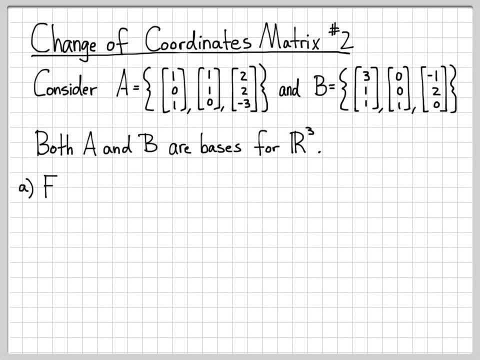 that we'll be working with in this example. So in part A, what we're going to do is we're going to find a matrix that takes us from vectors represented by bases B into vectors represented by bases A. So that's what we mean by this notation. right here, P will be. 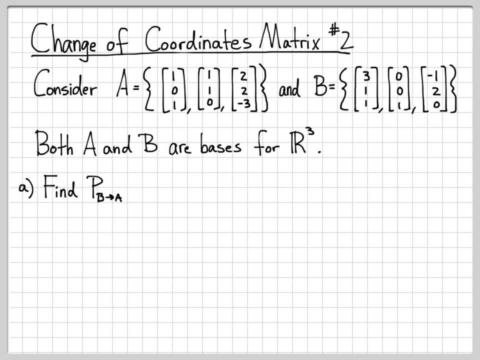 our change of coordinates matrix and it takes us from coordinates in the B bases to coordinates with respect to the A bases. We know in general how to do this. We need to form a matrix whose columns consist of the vectors in the starting bases. So we're going to start with vectors. 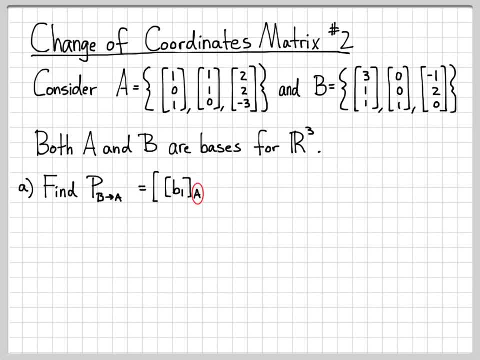 in the bases B, but we need to write them with respect to the bases we're going to. Since we're going to the bases A, we need to be able to write the vector B1. with respect to the bases A, We need to be able to write the vector B2, which is this vector right? 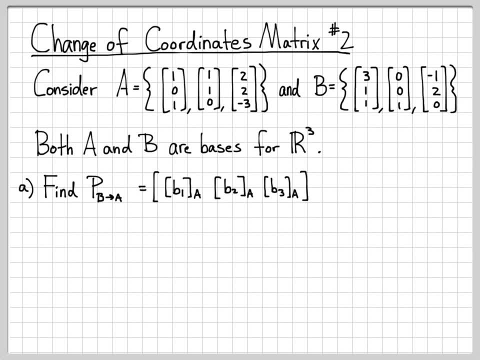 here with respect to the bases A, And also we need to be able to write B3, this vector, right here in the coordinates with respect to bases A. So this is what we need to do. We need to really do three independent computations to figure out what each one of these vectors are. So let's go ahead and start. 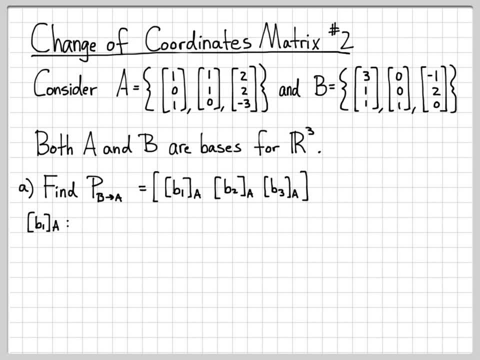 with the first one, How would I write vector B1 with respect to the bases A? So here is the vector B1.. It's the vector 311.. To write it in terms of coordinates in the A bases, to take a linear combination of these three vectors. So I need to be able to write 3, 1, 1. 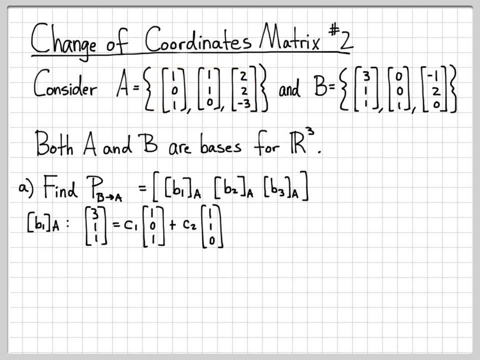 as a linear combination of 1, 0, 1, 1, 1, 0, and 2, 2, negative 3.. This is exactly what it means to write this vector with respect to the basis a. I need to find a linear combination of the. 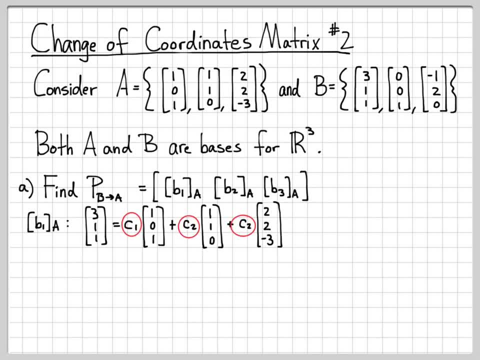 vectors in a and the components or the coefficients c1,, c2, and c3. tell me how to do this linear combination? So, if you look at this, I need to be able to write this vector as a linear combination of these three things, but I don't know what c1,, c2, and c3 are. So really I need to solve for. 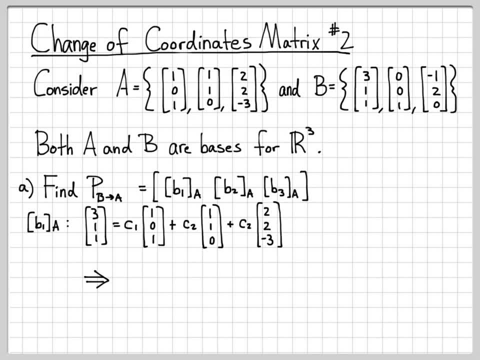 those unknowns, but that's pretty easy. This is just a system of equations so I can form my augmented matrix, like we always do in solving a system of linear equations. If I do that, I know I need to take linear combinations of these vectors and it needs to equal this. So this is. 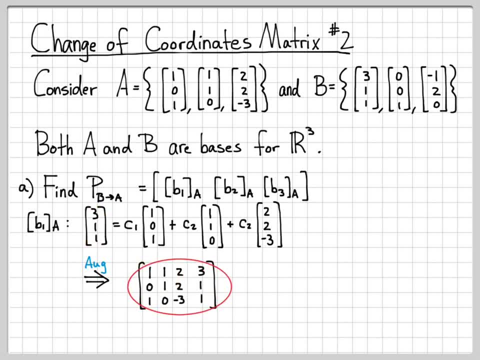 my augmented matrix right here. So this is the augmented matrix that I need to solve. We're not going to go through all the details. I have plenty of videos earlier in the playlist that walk through how to construct an augmented matrix, then perform. 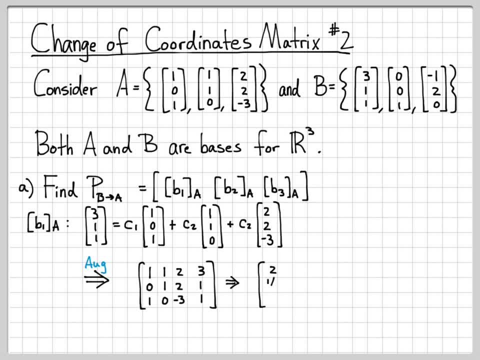 row operations to solve it. If we go through all those steps, what we'll find is that c1 is equal to 2, c2 is equal to a third and c3 is equal to one third. And I just noticed I had a little typo. 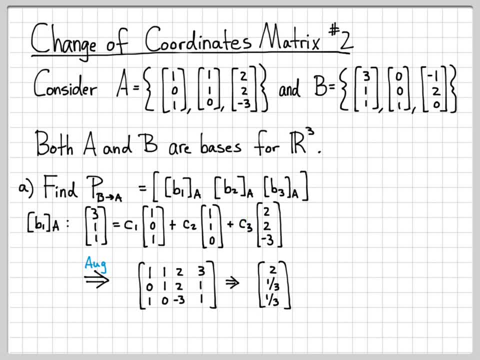 right there. That should obviously have been c sub 3, so I went ahead and corrected that. So this is how we can write the vector 3, 1, 1, as a linear combination of the vectors in a. So this right here, by definition is the vector b1. 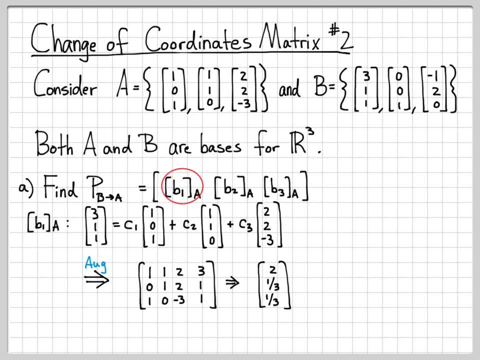 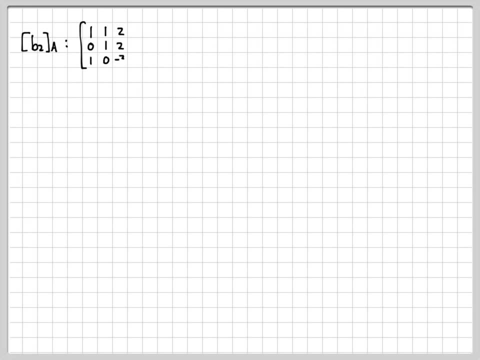 with respect to a. So we have solved for this piece right here. We now know the first column of our coordinate transformation matrix p from b to a. We need to do similar things for the other two vectors now. So let's go ahead and do those. We'll do those a little bit more quickly. We need 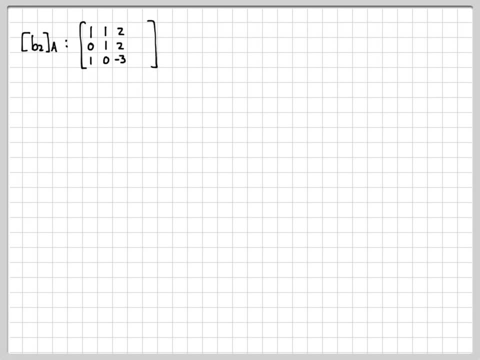 to be able to write the second vector, b2, with respect to a. This is the augmented matrix that I would need to solve. So if I do that and do all the row operations I would do to do this, I would end up solving for the coefficients c1, c2, and c3. 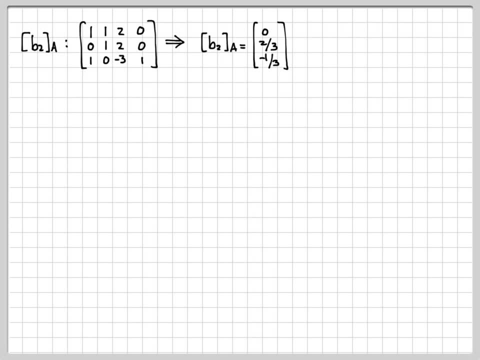 as 0, two thirds and a negative one third. So that is b2 written with respect to the a basis. And then, finally, similar thing for b3.. I need to be able to write b3 as a linear combination of the vectors in a, So I form my augmented matrix. This time, though, I put b3 right here. 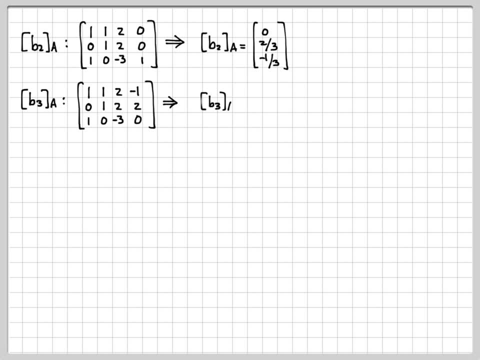 I do row operations, I do a linear combination of the vectors in a, So I form my augmented matrix. I do row operations And I solve for the coefficients to solve this linear system of equations. And I end up with this vector for b3 with respect to a. So I've solved for each. 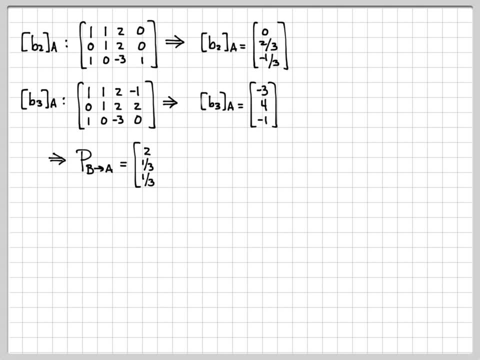 column in my coordinate transformation matrix. This was b1 with respect to a, This is b2 with respect to a And this is b3 with respect to a. So we have solved for a change of coordinates matrix that lets us multiply a vector written in b coordinates and transform it into a vector. 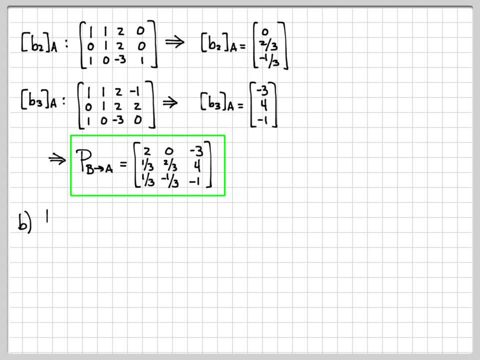 written in a. All right, that was part a. Let's do the opposite thing in part b. Let's find the change of coordinate matrix that takes us from coordinates with respect to the a basis to the b basis. So we know in general how to do this. I need to write a1 with respect to b. I need to write a2,. 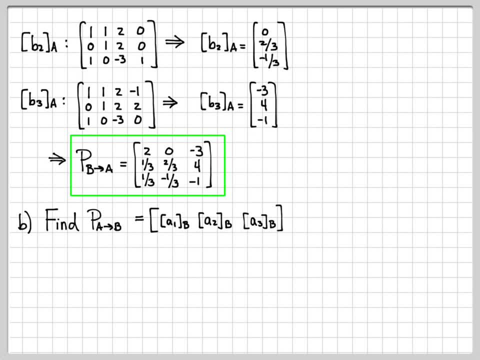 the second column of my basis with respect to b, And I need to write a3,, the third vector in the basis a with respect to the basis b. So again, what does this mean? I need to solve three systems of equations To find a1,, I need to be able to write the vector a1, which is: 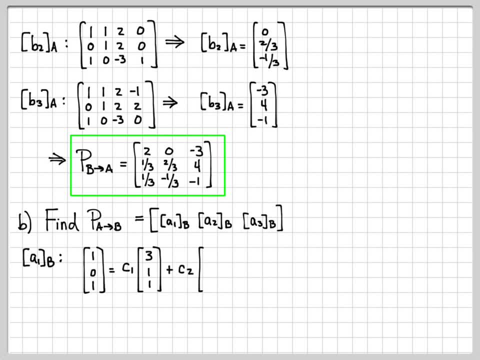 1, 0, 1, as a linear combination of the vectors in the basis b. So these are the vectors in the basis b. I'm taking a linear combination of them. I'm trying to find c1 and c2 and. 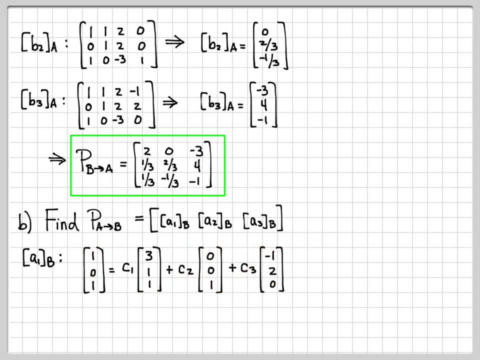 c3, such that this equation is true In general. how do I solve an equation like that? I form an augmented matrix And I solve that augmented matrix To get the unknowns c1,, c2, and c3.. So if I can solve this augmented equation, I get c1,, c2,. 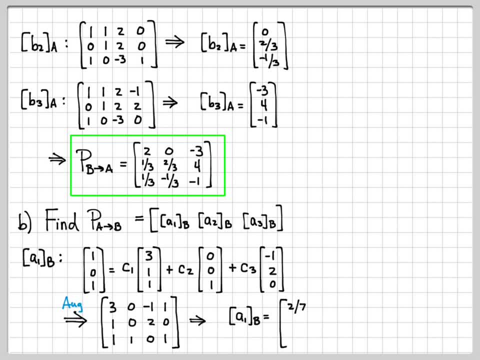 and c3. Again, skipping the details because we've done this many times previously. in the playlist of these videos I would find that c1 is equal to 2 sevenths, c2 is equal to 5 sevenths and c3 is equal to a negative 1 seventh. So this is the vector a1 written in terms of the. 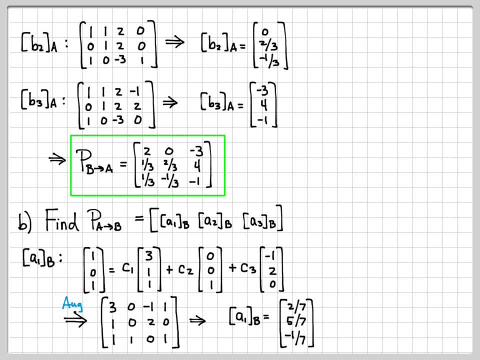 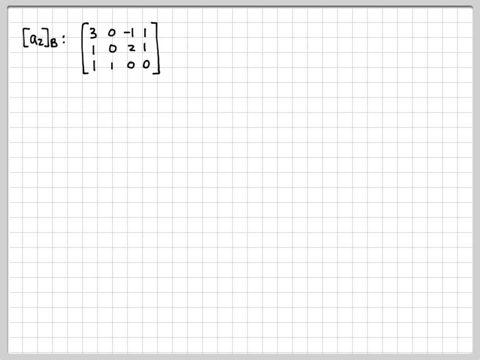 coordinates with respect to basis b. We can keep doing this And we'll go through this a little quickly now. To find a2 with respect to b, I solve this augmented matrix which gives me the vector a2 with respect to b of 3 sevenths, a negative 3 seventh and 2 sevenths, And then finally to write: 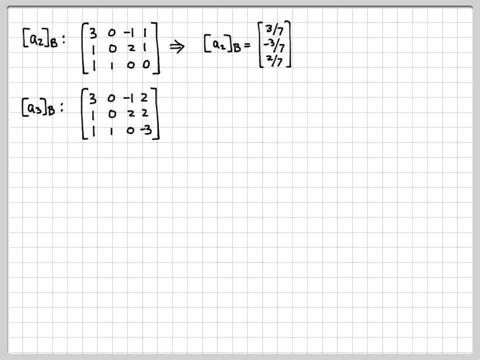 a3. with respect to b, I solve this augmented matrix, which is just a system of equations, to yield this vector. So I've solved for all three columns of my coordinate transformation matrix. All of them have a 1 seventh in them, so I'm going to pull that 1 seventh out front And 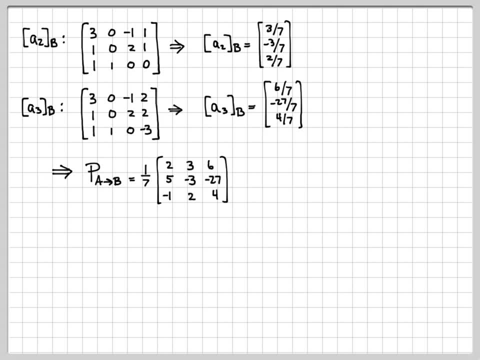 then I can write my change of coordinates matrix nicely like this. So this is the change of coordinates matrix that takes me from vectors written with respect to basis a into vectors written with respect to the basis b. Let's go ahead and do a little check here. Let's 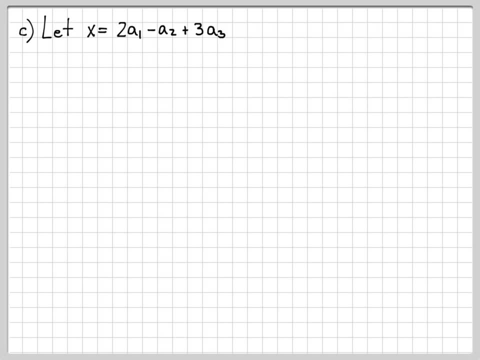 say, we're dealing with the vector x, which can be written as 2a1 minus a2 plus 3a3.. So what does that mean? That means we have a vector representation with respect to the a basis of 2, negative. 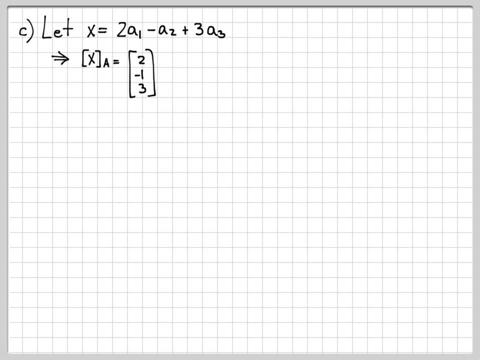 1, and 3,, because x, as written right here, has 2a1s, It has minus 1a2, and it has 3a3.. So, by definition, this is how we would write x in terms of the basis a. Let's go ahead. 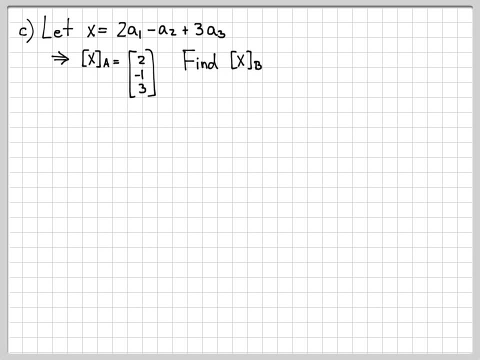 and find x of b, Let's write x in terms of the basis b, Since we've computed our change of coordinates matrix that takes us from a to b. I can do that pretty easily. All I need to do is take my vector written with respect to the coordinates in a and multiply it by. 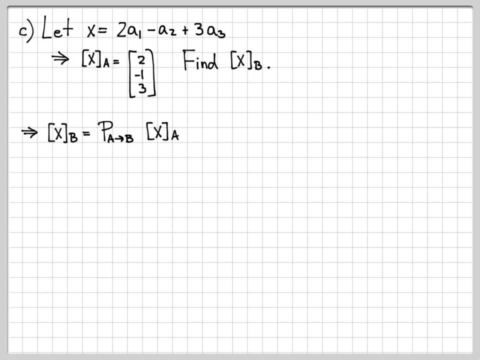 my coordinate transformation matrix that takes me from a to b. So if I can just do this matrix vector multiplication, I can do this transformation very easily. If you go back a page and look at what our coordinate transformation matrix was that took us from a to b, we had this: 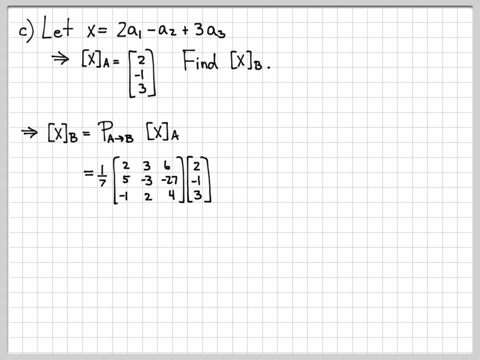 In the problem where we figured out when a and b happened. we had a matrix that took us from a to b, and we had a matrix that took us from a to b, and we had a matrix that took what the representation in the A basis was of the vector. It was this, And if we just do this, 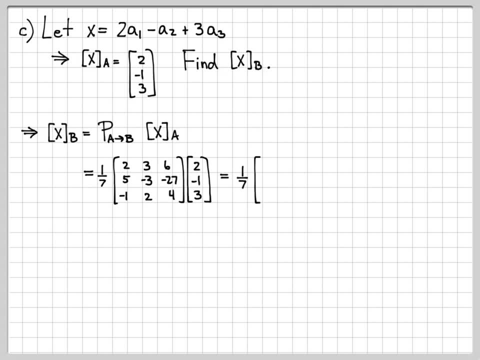 multiplication, we obtain this answer: 1, 7th, 19, minus 68, and 8.. So this is how we would write the vector x with respect to the basis B. Let's do a little check. I should be able to take this.